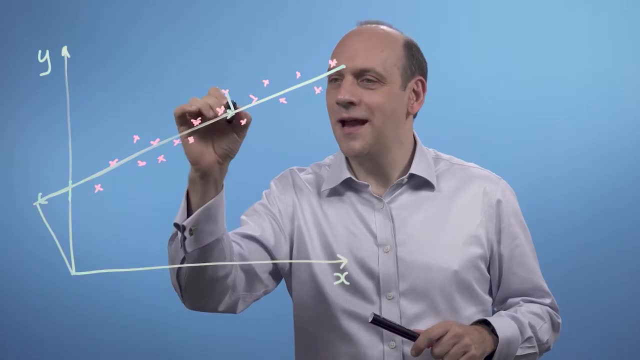 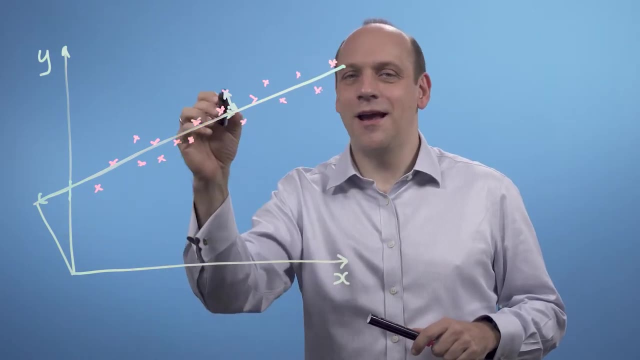 far along the line there and he's this far away from the line. So I've got two dimensions here: How far I am along the line and how far I am from the line And these guys. they're all slightly different distances from the. 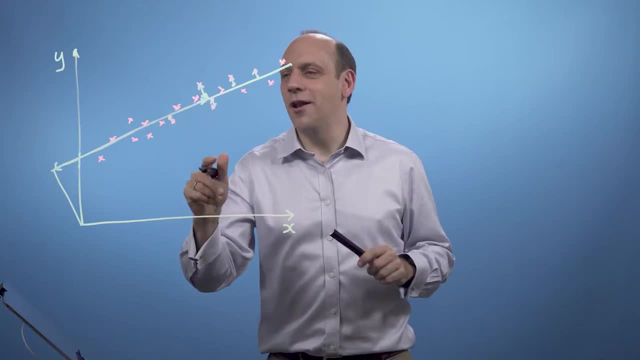 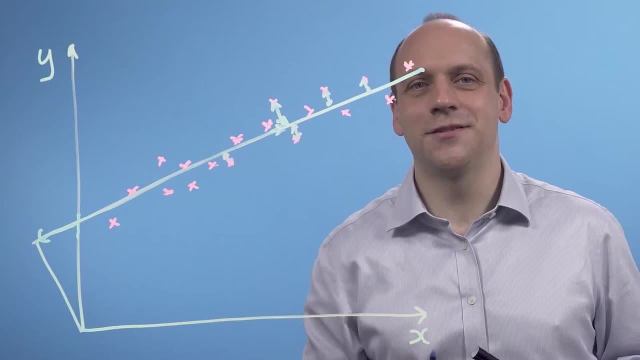 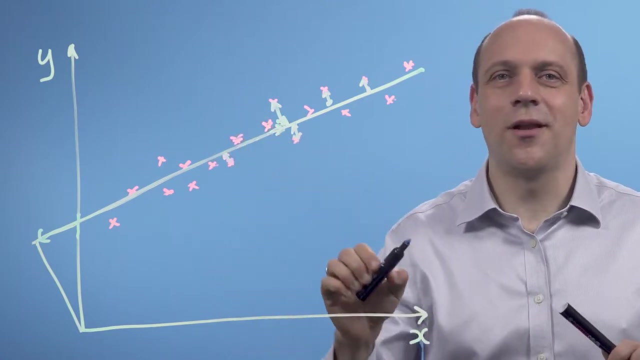 line. Now there's a little bit of an argument in stats as to whether we do the distance that way vertically or that way as a projection for the distance from the line. But it's sort of a theoretical argument. But notice that this distance from the line is effectively. 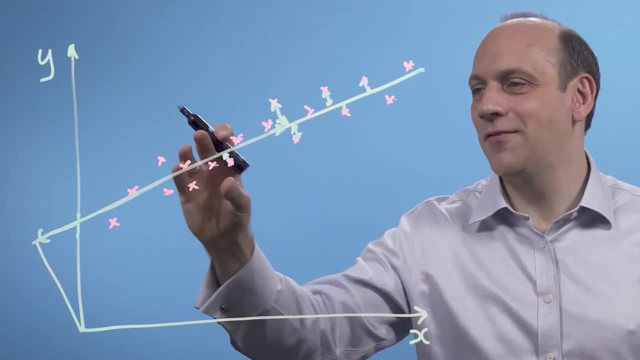 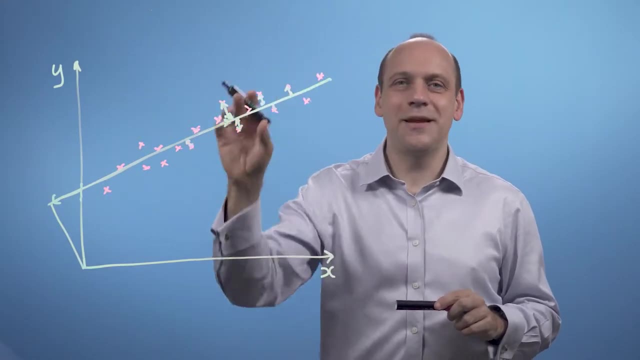 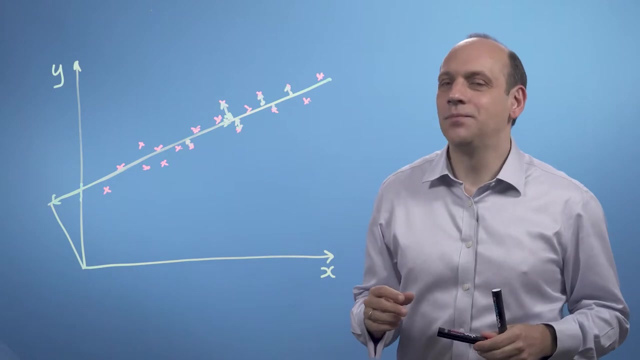 a measure of how noisy this data cloud is. If they are all tight on the line, they're all very small distances away, And if they were all quite spread, they'd be quite big distances away. So this distance from the line-ness is, in fact, the noise, And that's. 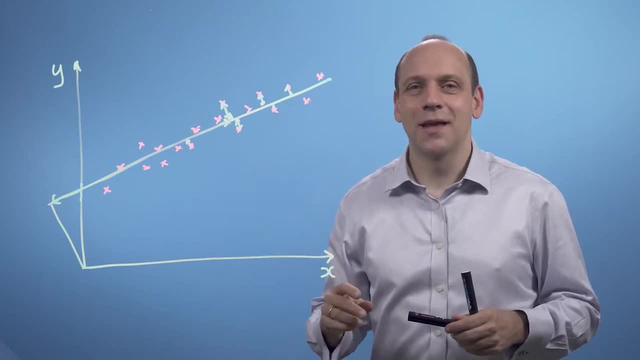 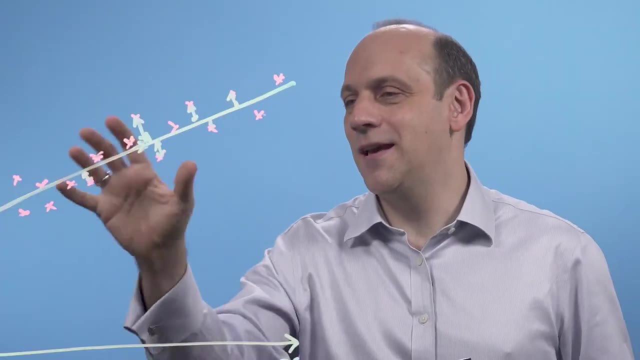 information that isn't very useful to us. so we might want to collapse it, Except that that noise dimension tells me how good this line fit is. If the best fit line was all skewed, was all wrong, I'd get a much bigger numbers for the noisiness. 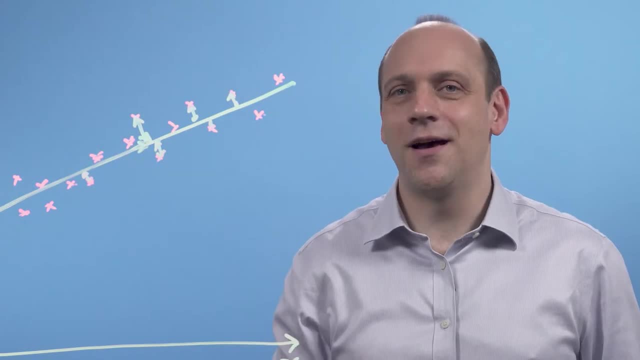 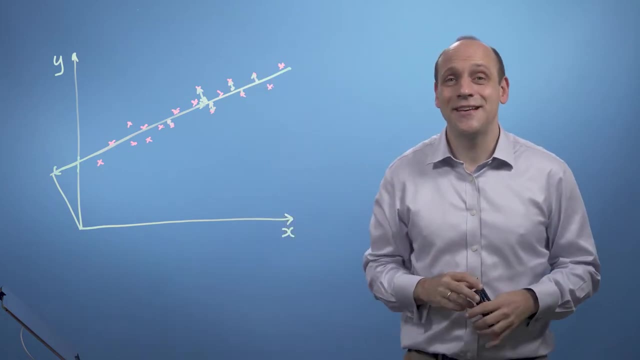 And if the best fit line was as good as possible, I'd get the minimum possible number for the noisiness, So that noise dimension contains information that's going to tell me how good my fit is. So when I'm doing data science, it tells me how good my fit to my data is. 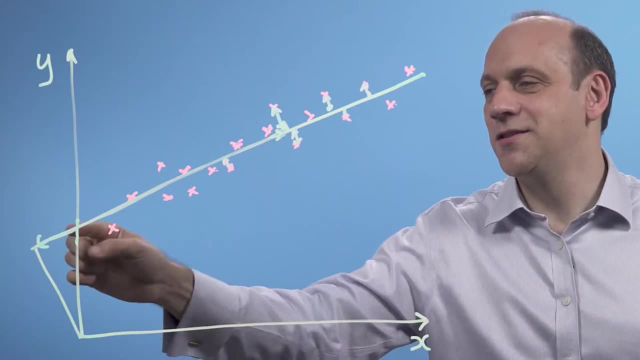 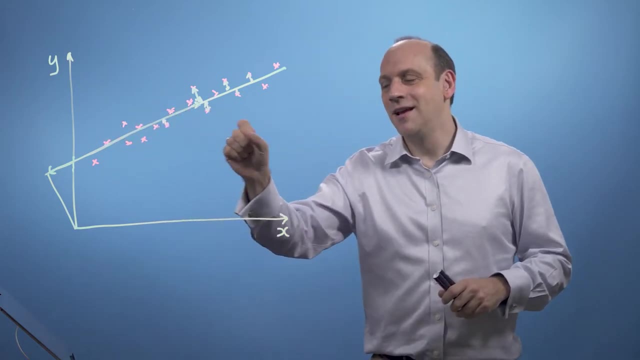 And the way I've defined these two directions- along the line and away from the line- they're orthogonal to each other. So I can use the dot product to do the projection to map the data from the xy space onto the space in the y space. So that's the big difference there. 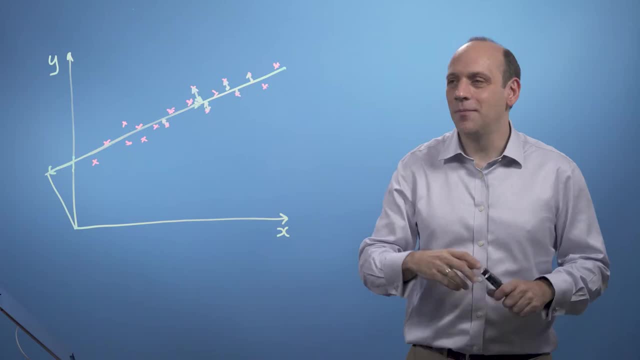 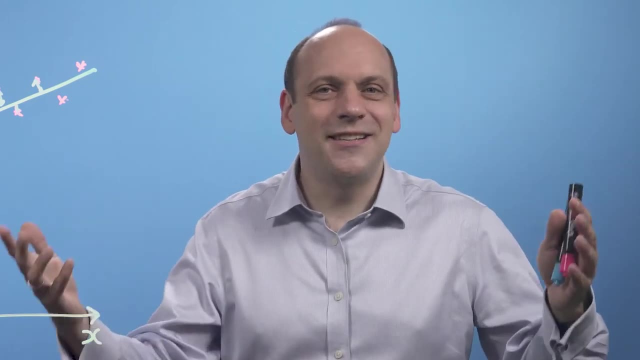 is the line, along the line and away from the line, which is what we learned to do in the last little segment. Now, if we're thinking about a neural network in machine learning that recognises faces, say, maybe I'd want to make some transformation of all the pixels in a face into a new basis. 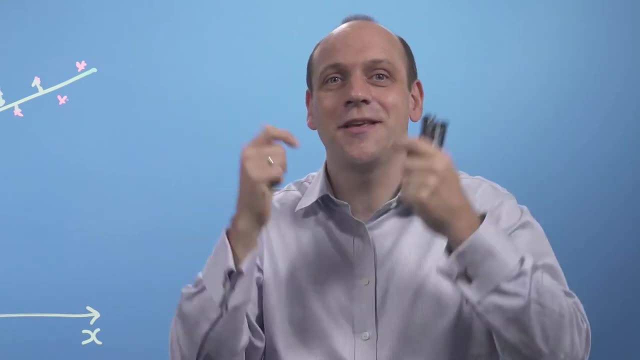 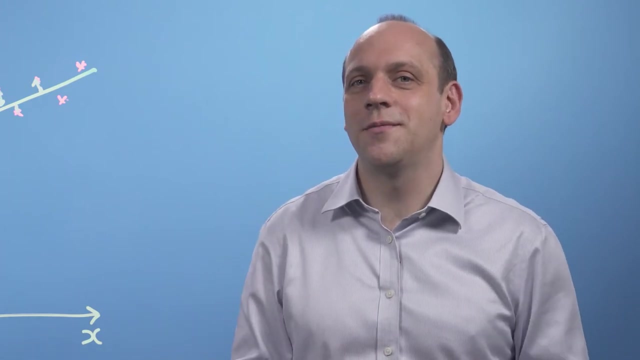 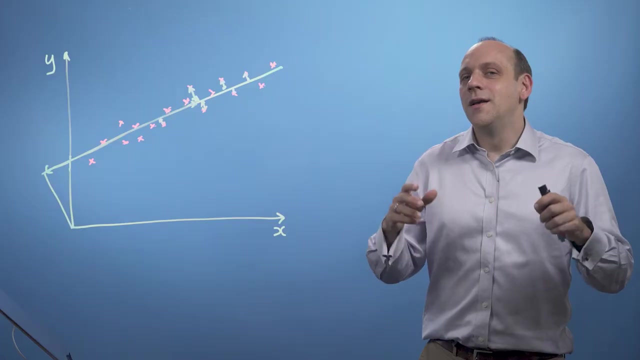 that describes the nose shape, the skin hue, the distance between the eyes, those sorts of things, and discard the actual pixel data. So the goal of the learning process of the neural network is going to be to somehow derive a set of basis vectors that extract the most information rich features of the faces.